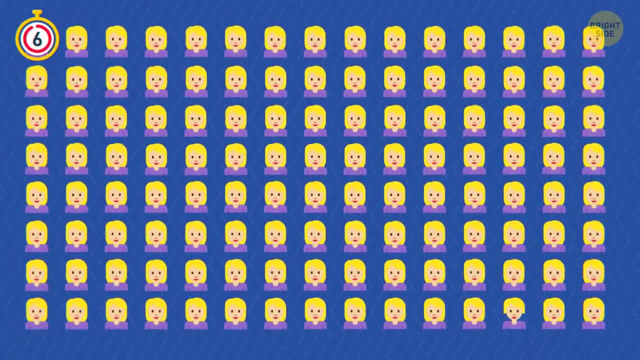 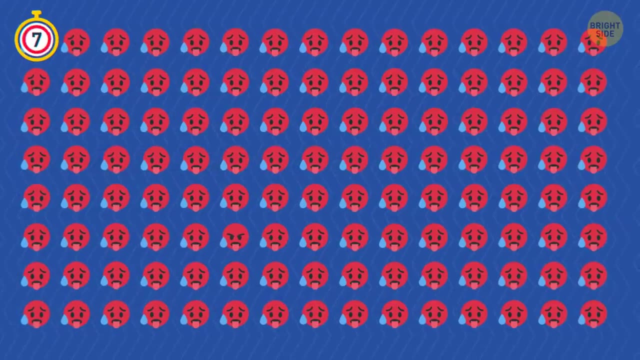 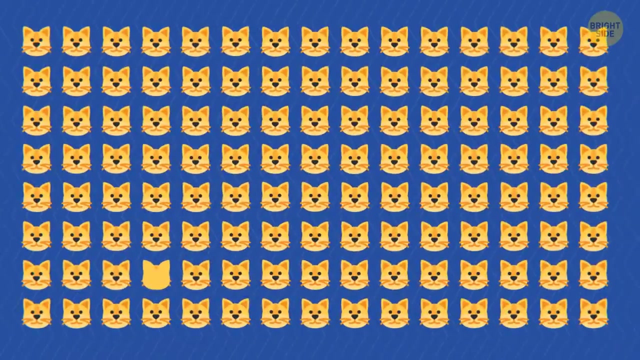 Which person is different from the others? Right, this one with shorter hair. Try to figure out which emoji is the odd one. The one at the bottom. Not only does it feel hot, it also looks pretty angry. I challenge you to find a cat that is different from the rest. 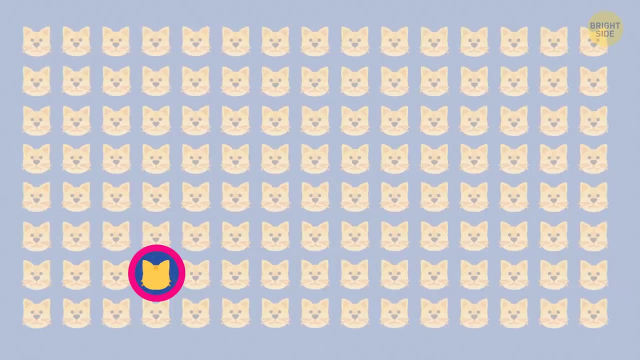 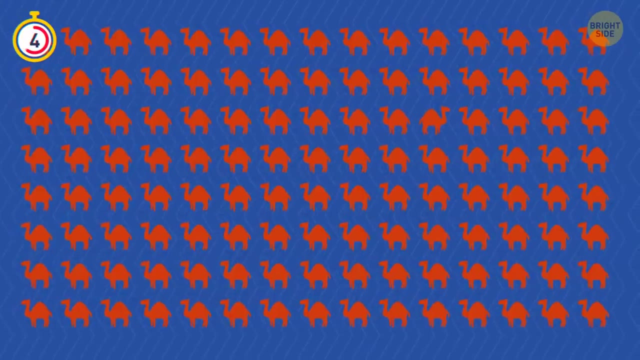 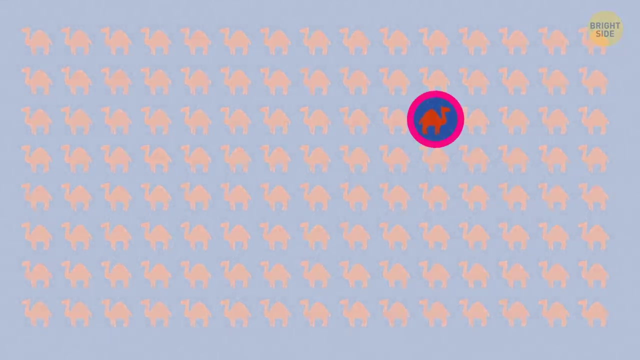 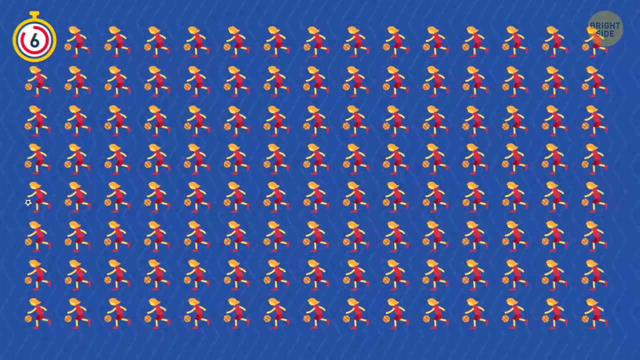 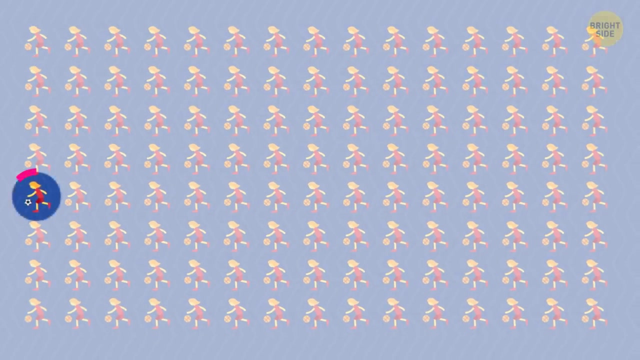 Right, it's the one closer to the bottom, facing away from you. Which image is the odd one? This little rebel is turned in the opposite direction. Have you noticed anything wrong with this picture? The ball, It's for playing soccer, not basketball. 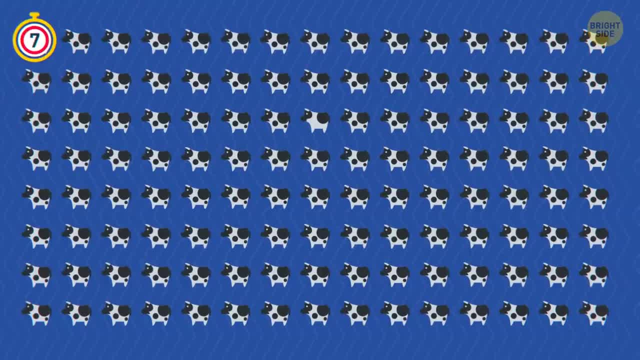 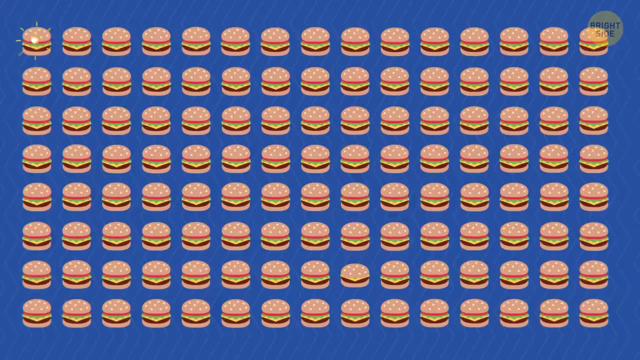 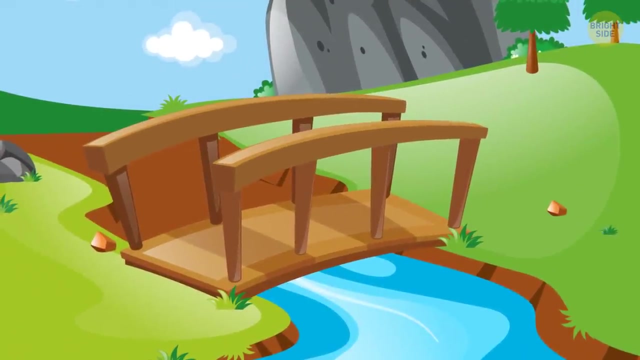 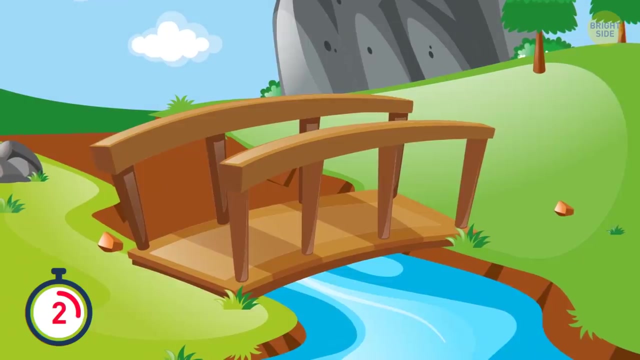 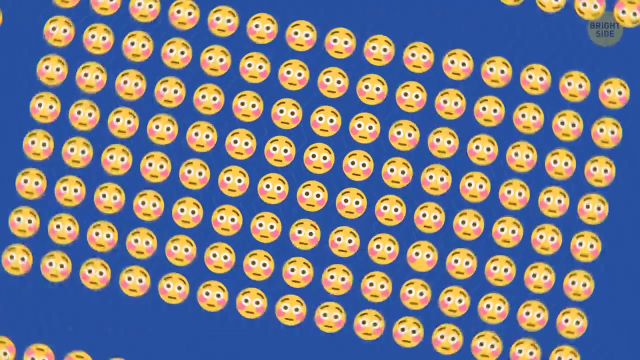 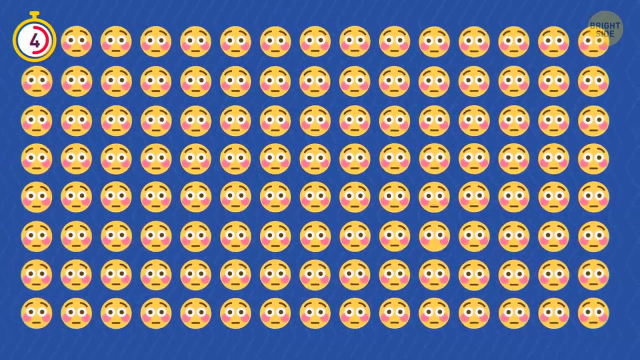 Which cow is different from the others? This one, The one below This, is definitely the one. So what's next? How about each unfortunately different emoji? It's the river. it just seems to disappear under the bridge. Which emoji is the odd one? 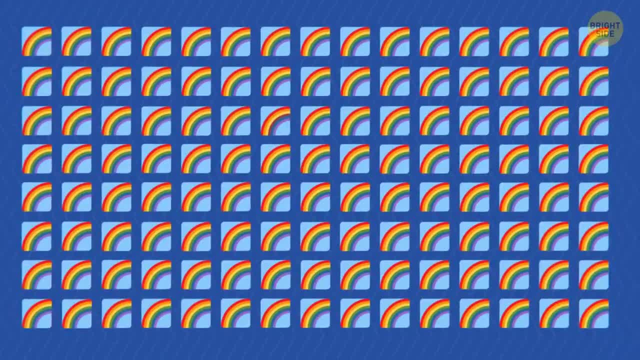 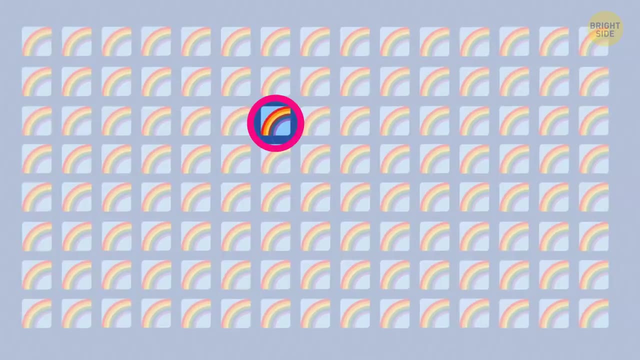 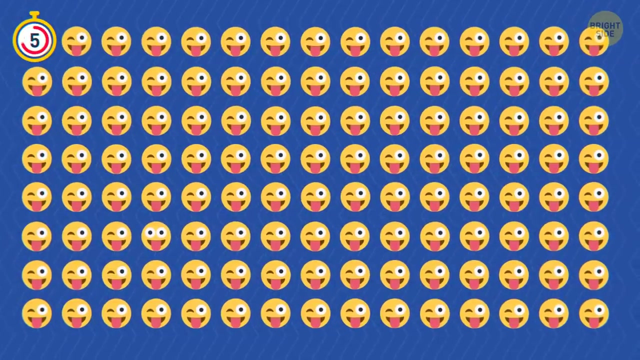 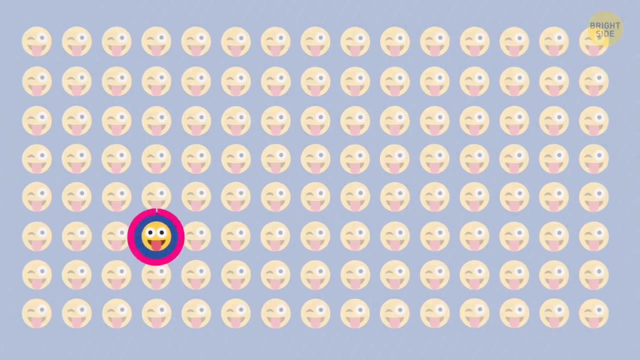 The one missing its mouth. There's something that doesn't seem quite right in this picture, but what? Its colors are a bit messed up. Which emoji is different than the others? It's the one with both its eyes open. These smiley faces look cool. 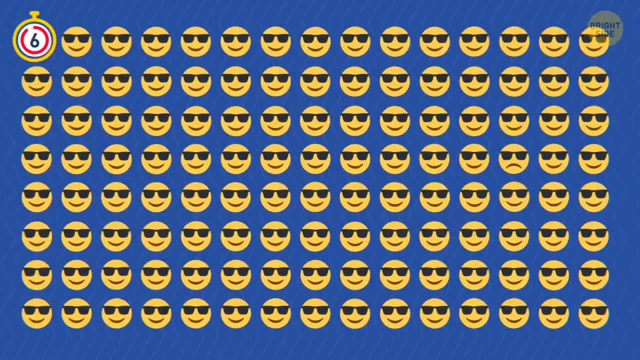 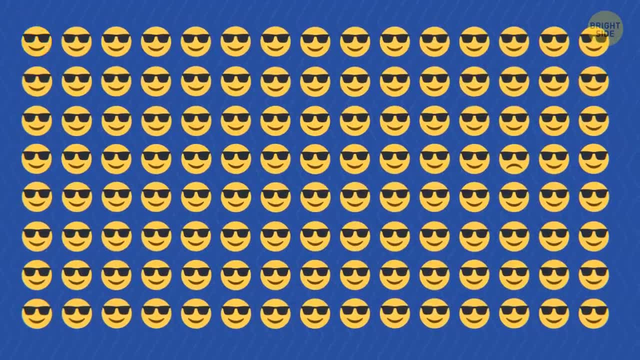 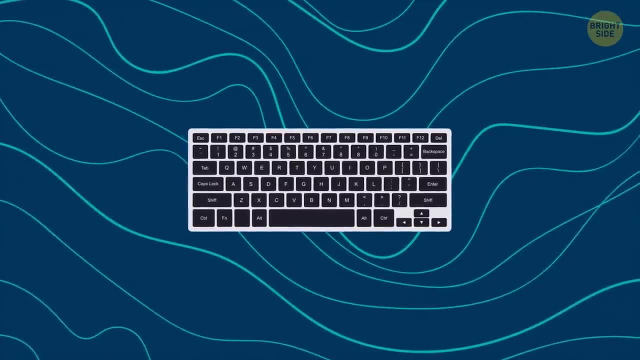 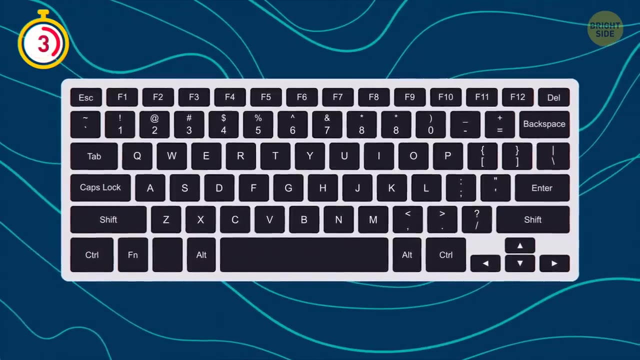 It's the one with both its eyes open. These smiley faces look cool, All but one. This emoji isn't actually all that smiley. There's something wrong with this keyboard. Can you figure out what exactly? There are two eights on it. 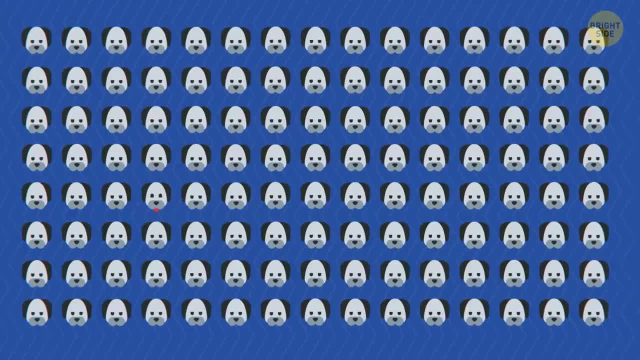 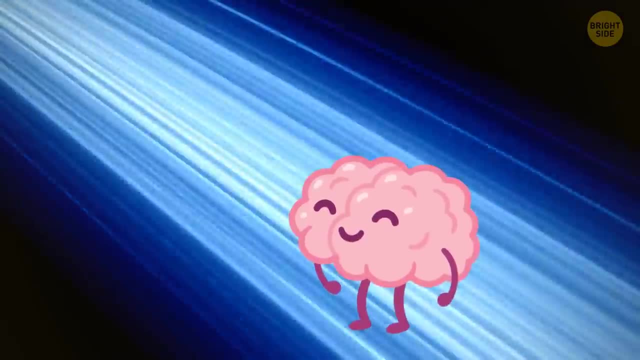 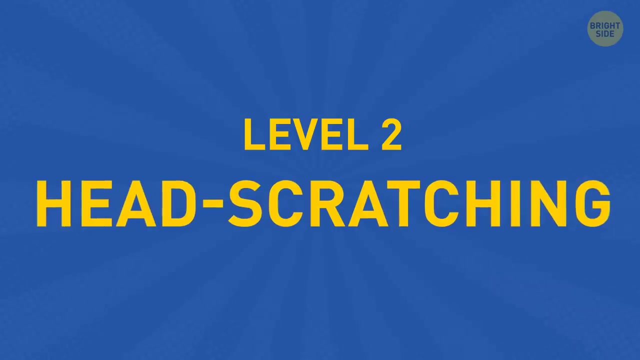 No, nines. Which pooch is the odd one? This doggy seems to be friendlier than the rest. This level didn't seem too hard to me, but are you up for some real challenge? Level 2. Head-scratching. 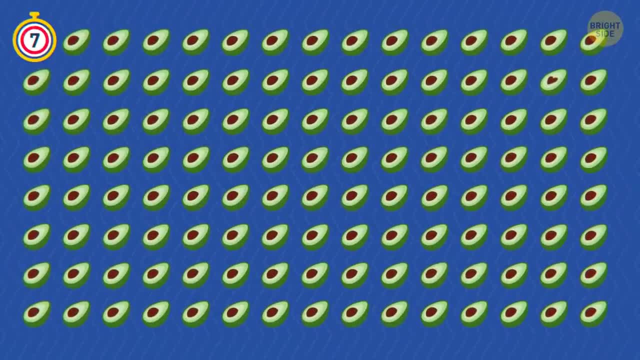 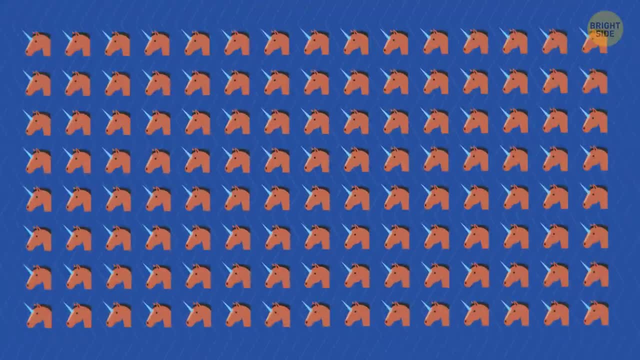 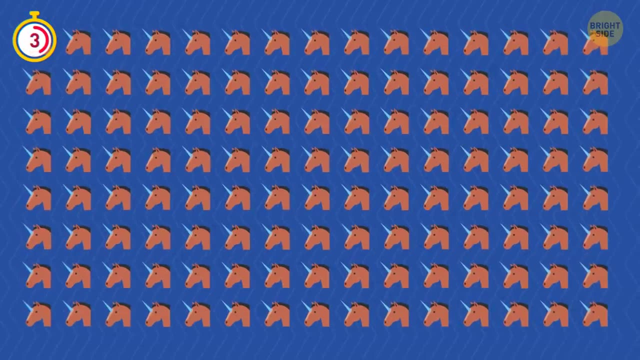 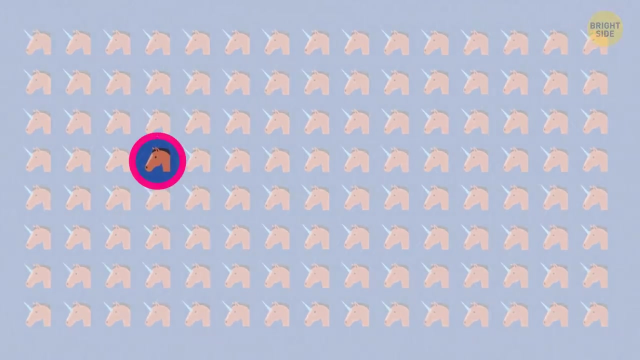 Which emoji is different than the others? It's the pet cat. Find the odd avocado. Find the odd avocado. This little guy is just a wannabe. It isn't a unicorn, It's a horse. Shoulda wounded, your pig하고. 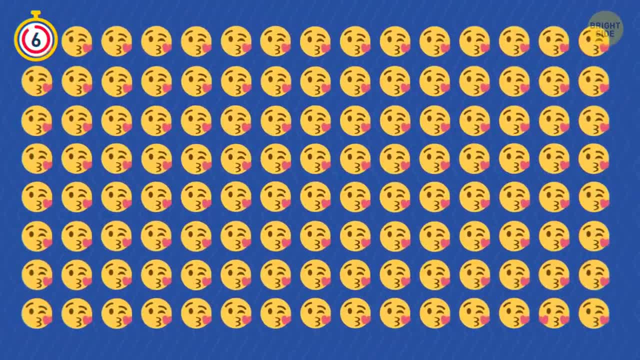 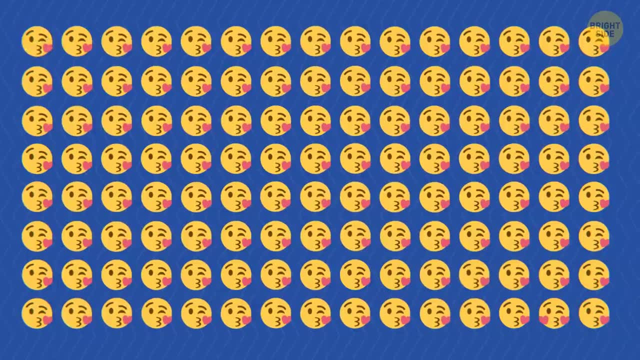 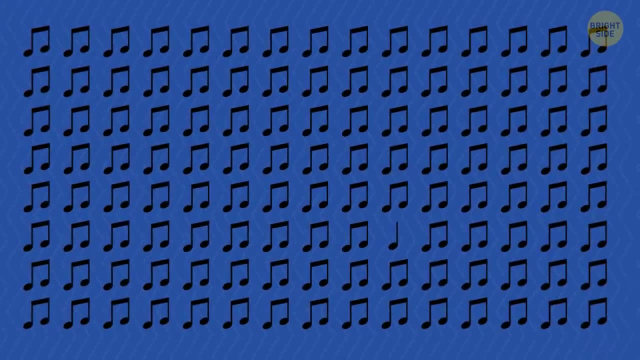 Can you find the odd emoji? I can find an old one. Oh yeah, Can you find it? The one at the bottom seems to be even more in love than the rest. One of these music notes is different. Which one? Ah, now I see it. 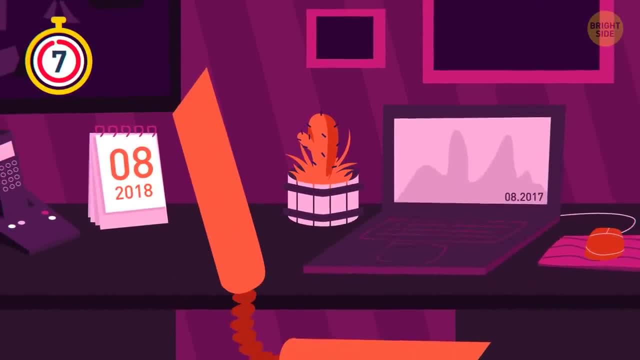 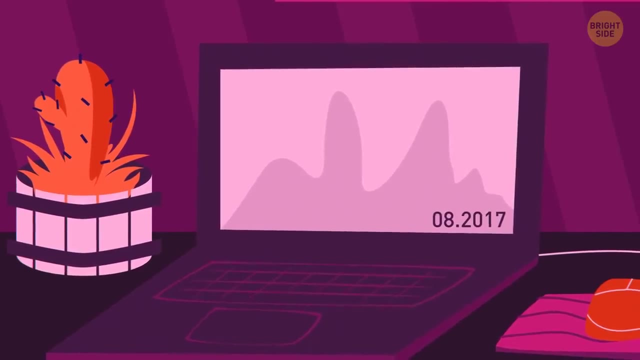 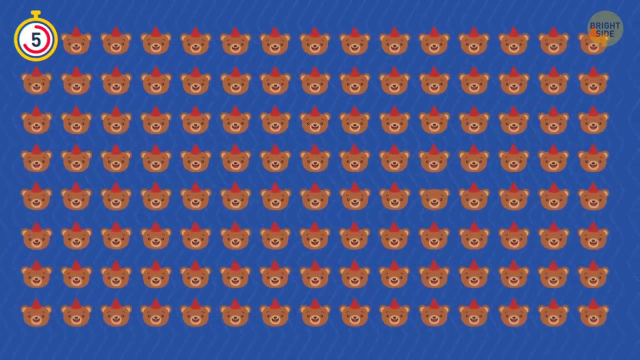 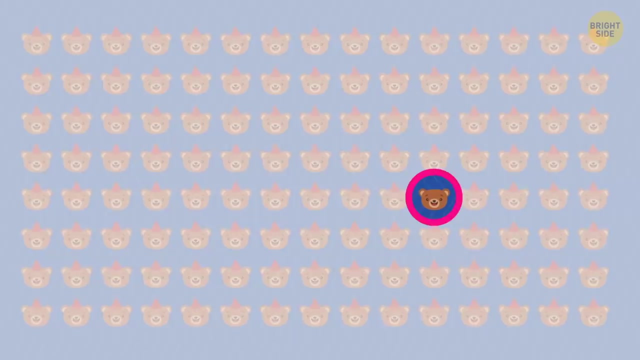 What's wrong with this picture? The calendar's claim it's August 2018.. But the computer is sure it's still August 2017.. Can you spot a teddy bear without a hat? Here it is. There's something strange about this picture. 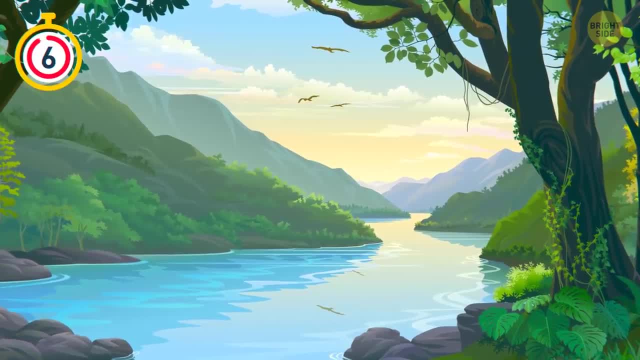 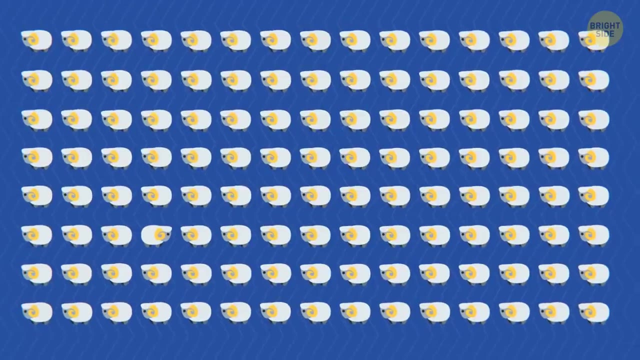 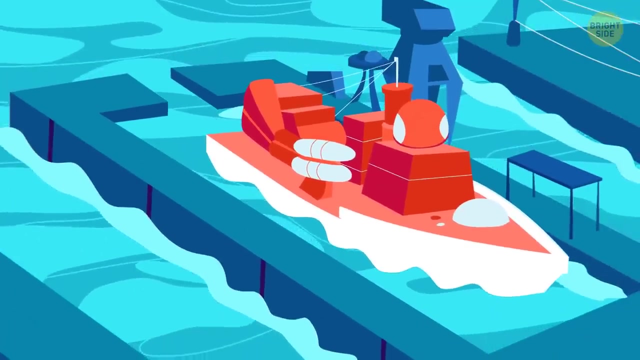 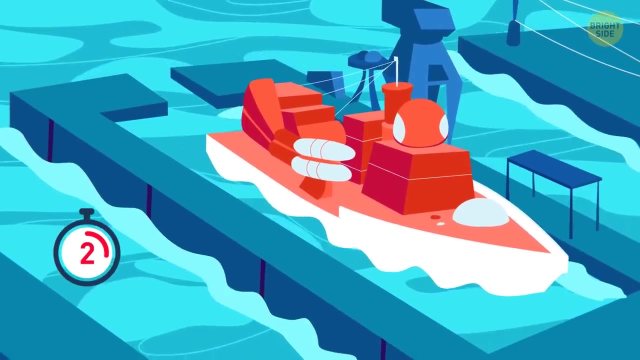 But what exactly? One of the birds doesn't have a reflection. Ew, creepy. What sheep is different from the others? This one, Don't? you think there's something wrong in this image? I've got only one question: How did this massive ship get inside? 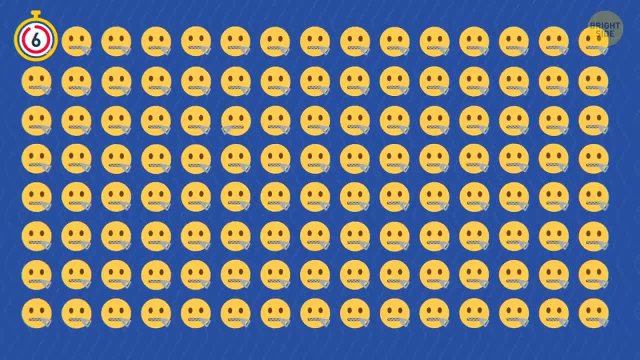 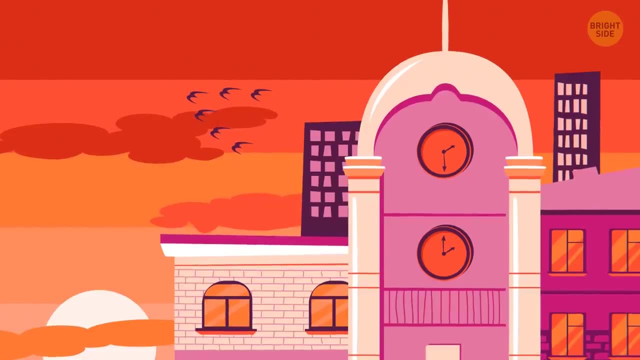 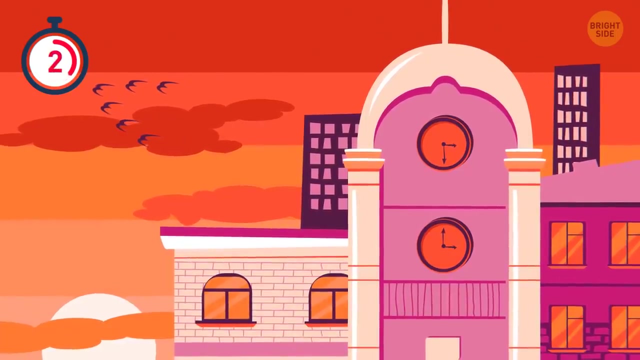 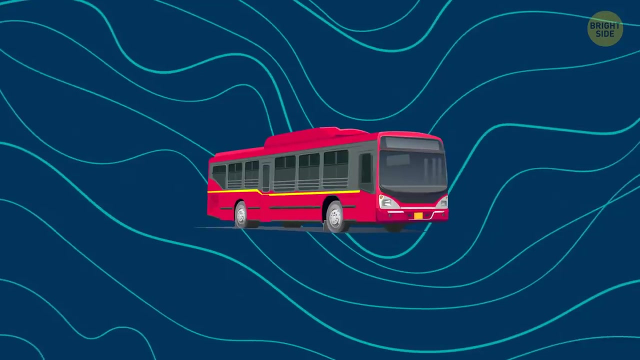 Which emoji is the odd one? This one: Its zipper, is on the left, not on the right. Look at this picture closely and find what's wrong here. The clock shows different time- And now find two things missing in this image. 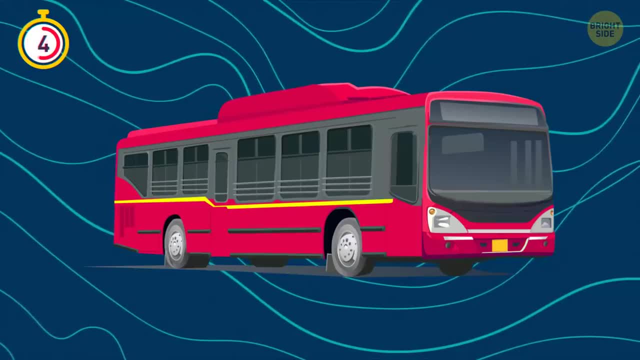 The clock and time are following the same size. What is the problem? The clock and time are fake. The clock and time are a lie. The clock and time are not real. The clock and time are fake. The clock and time are fake. 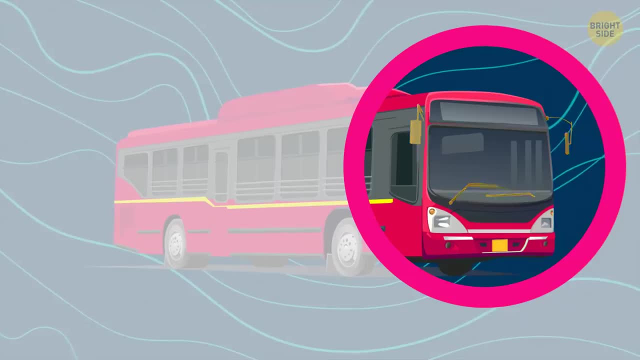 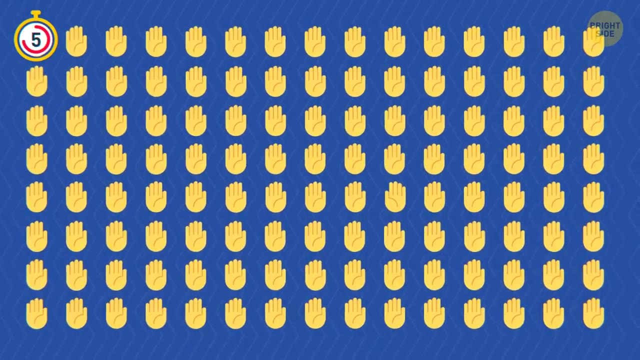 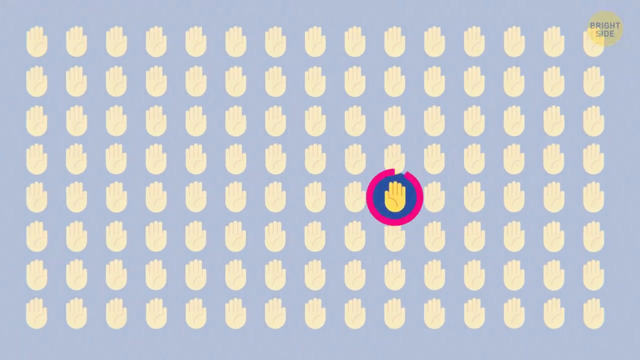 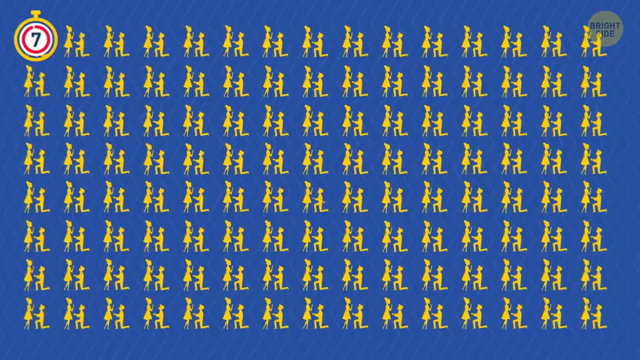 The bus lacks side mirrors and windshield wipers. Try to figure out which emoji is the odd one. This is a left hand, while the others are right ones. Which couple is different from the others? The one in the middle? There, the man is still hiding the ring behind his back. 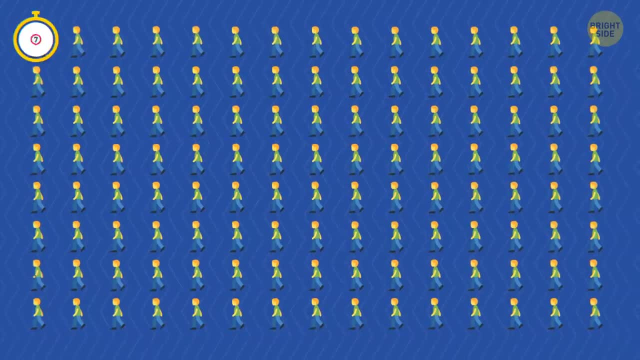 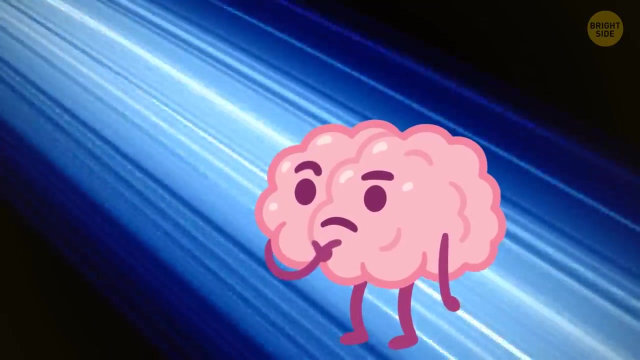 One guy is somehow different from the rest. Which one? It's the guy wearing a watch on his wrist. To tell you the truth, I even paused the video once or twice to figure out the answer. But there's still level 3 ahead. 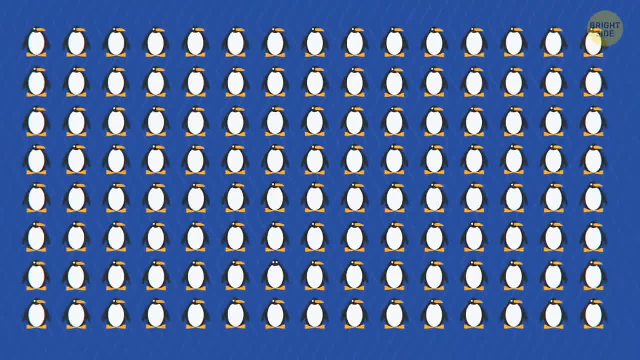 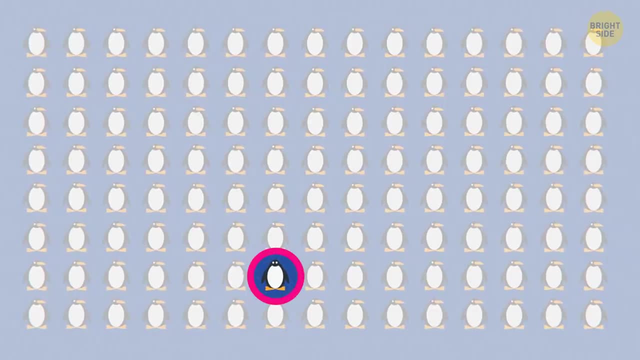 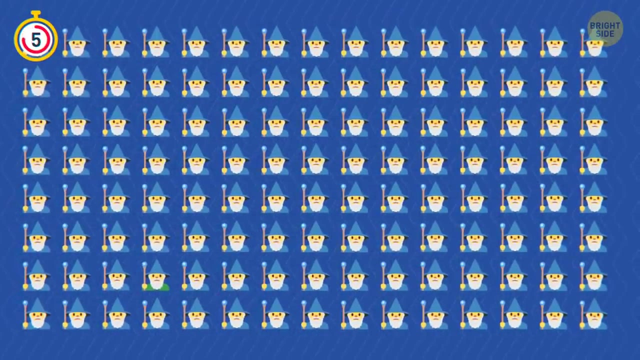 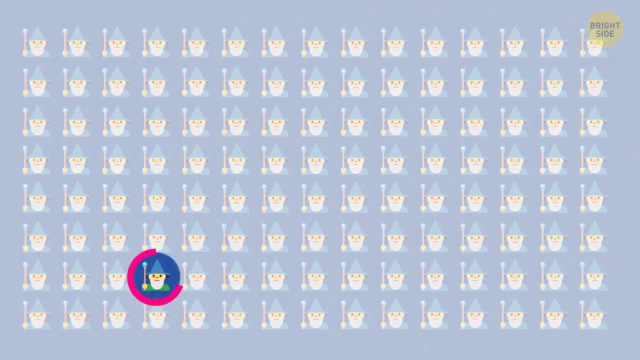 Level 3. Mind-boggling: Find the penguin whose bill is missing. Here it is. Now I see why this level is called mind-boggling. Which magician is different from the others? Look at this one. His robe is not blue but green. 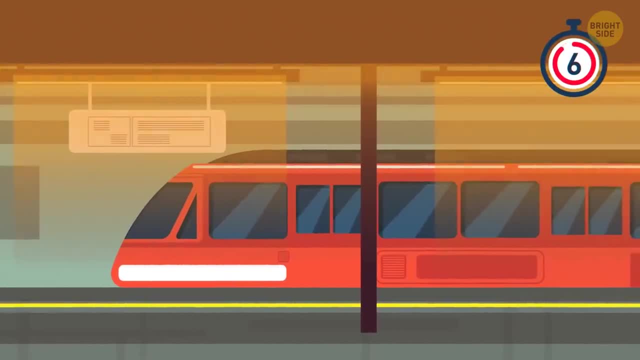 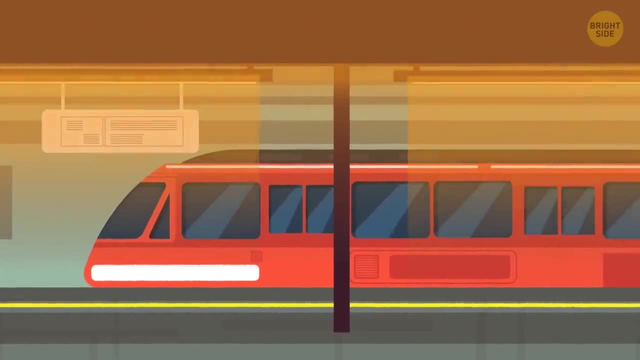 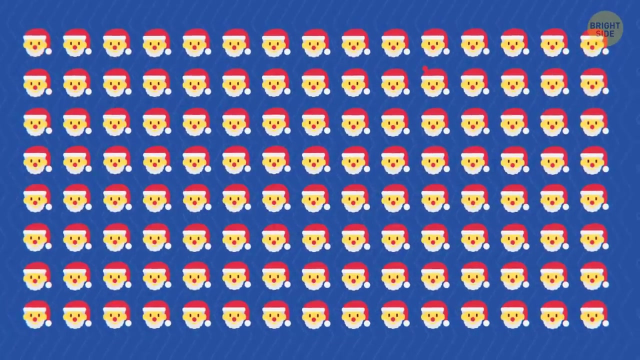 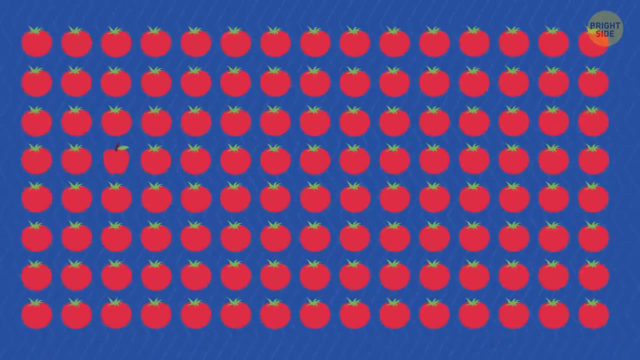 What's wrong with this picture? Electric trains have doors on both sides of the car. How fast will you find an extra pom-pom? This red ball is neither a nose nor a pom-pom. Wow, Can you spot an apple in this image? 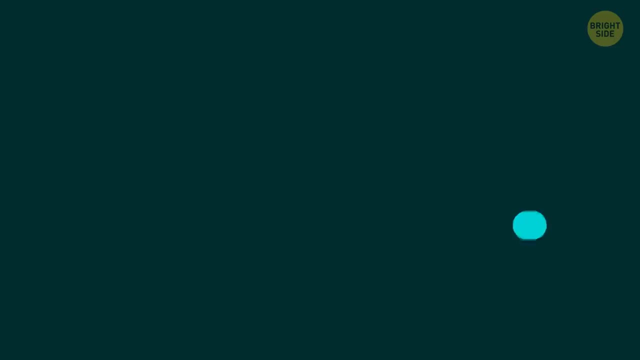 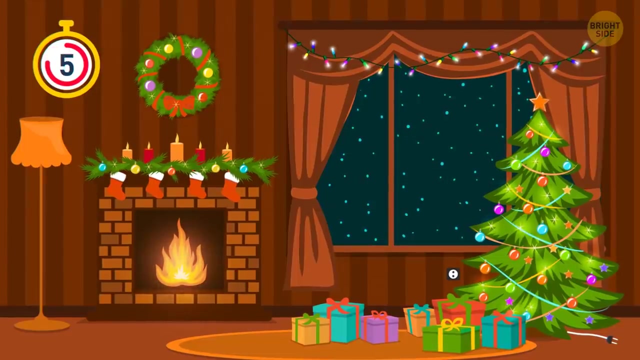 Ah, this is where it's hiding. Something is wrong in this picture, but I can't figure out what exactly. What's wrong? The fairy lights on the tree are shining, but they aren't plugged in. Which emoji is the odd one? 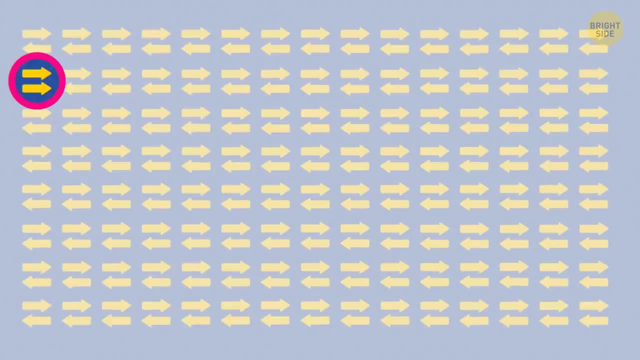 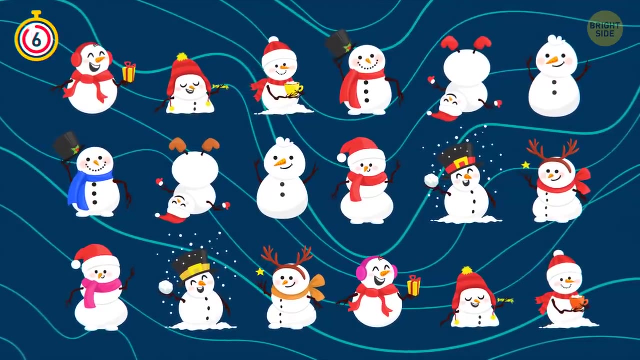 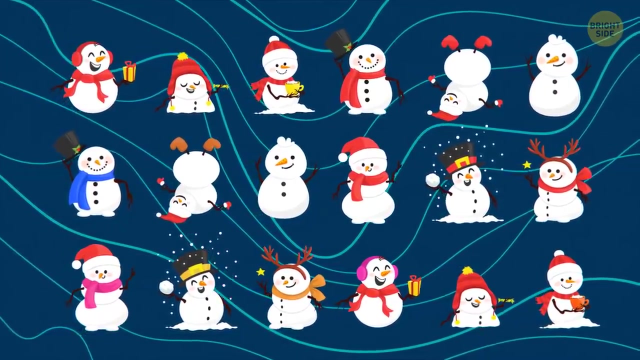 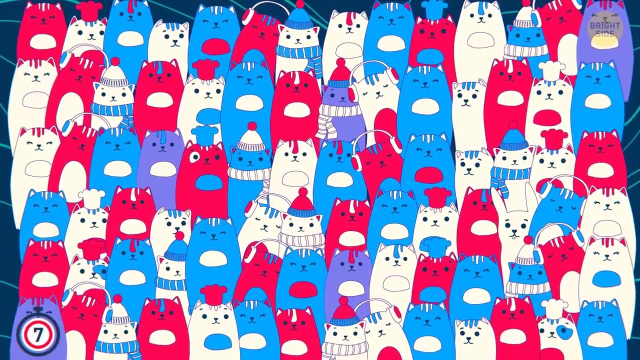 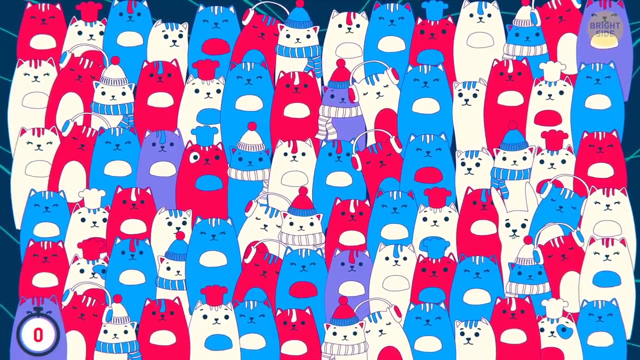 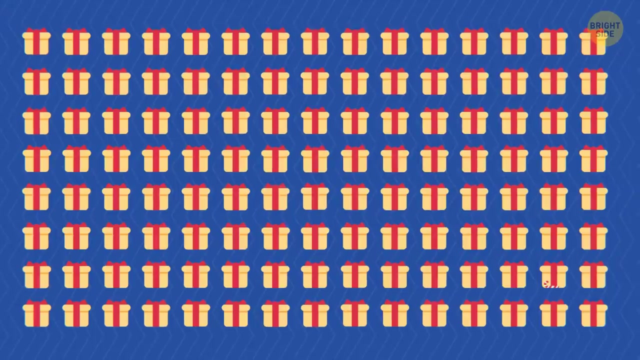 Unlike the others, these arrows are all pointing in one direction. Find two identical snowmen as fast as you can. Here they are the coolest ones. Can you spot a rabbit among these cats? This bunny is a guru of disguise. A candy cane is hiding among these gift boxes. 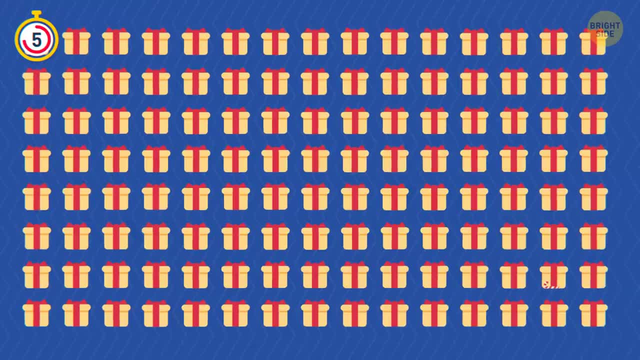 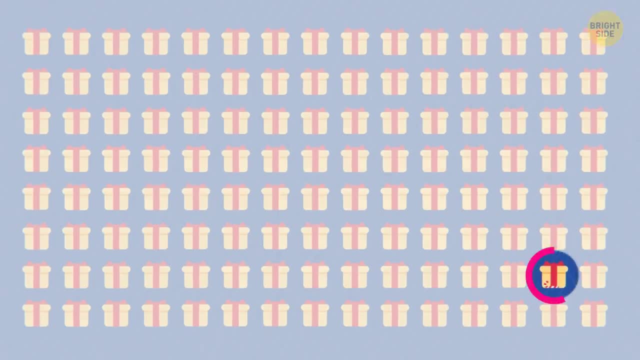 Do you see it? Can you spot a rabbit among these cats? This one is neither a nose nor a pom-pom. How fast will you find an extra pom-pom? This one is neither a nose nor a pom-pom. Nice try, but I'm too attentive to fail that. 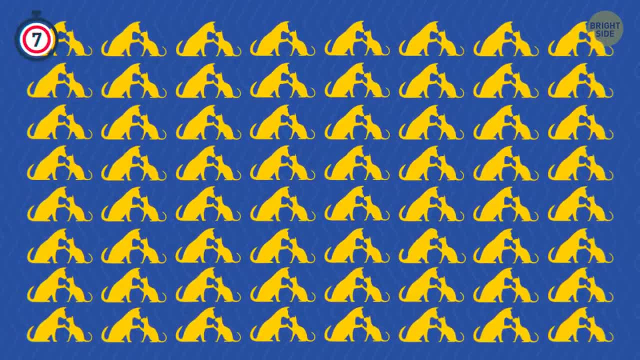 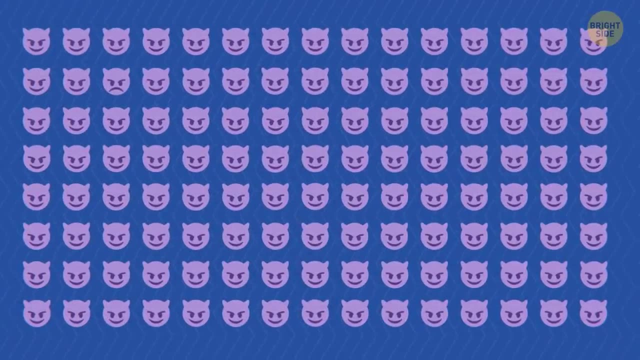 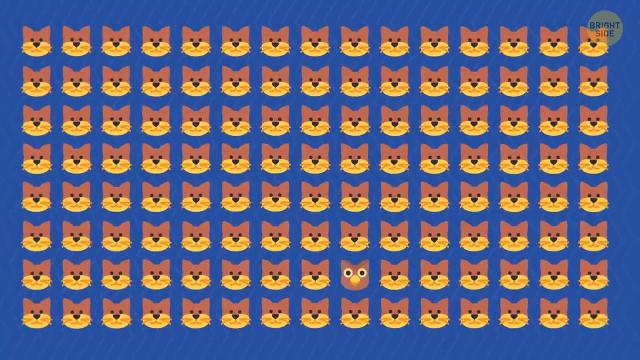 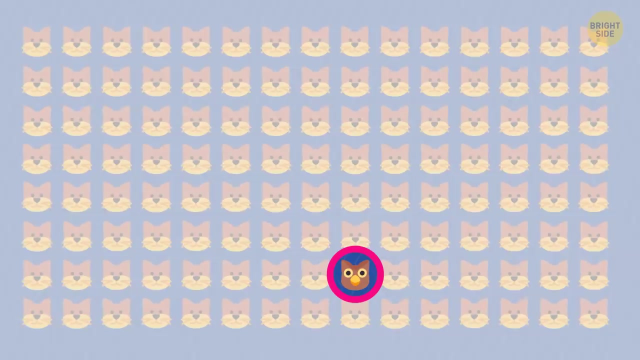 Which image is different from the rest? This dog is definitely a different breed. Find the odd emoji. This guy is way more evil than the others. One cat is somehow different, but can you figure out which one? it is? This one, because it's not a cat but an owl. 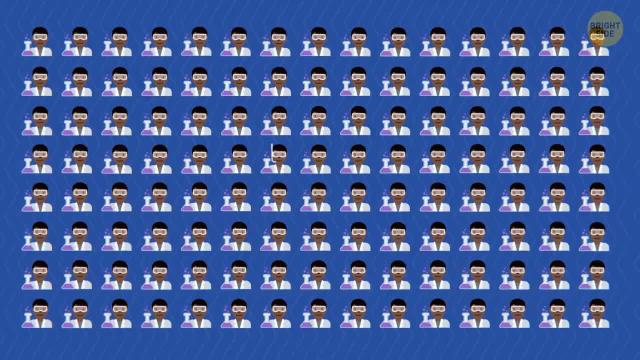 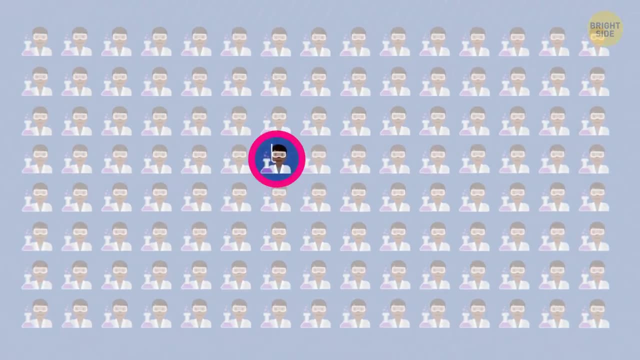 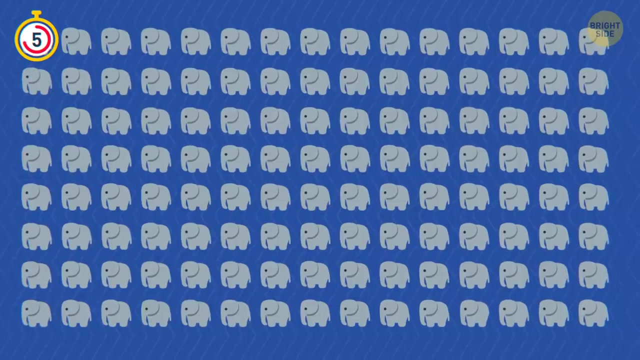 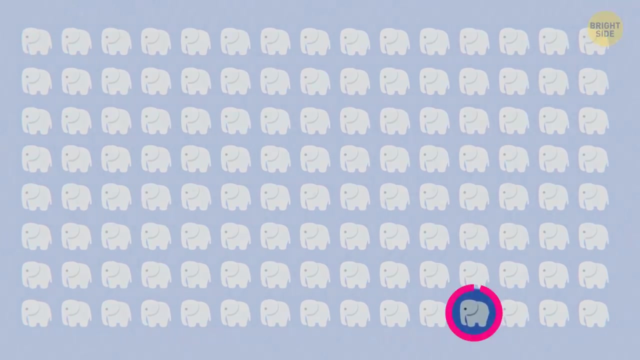 There's something wrong with this cat, There's something wrong in this image, but to figure out what, you need to be very attentive. This guy is wearing swimming goggles. One elephant is different from the others. Which one? The one at the bottom. 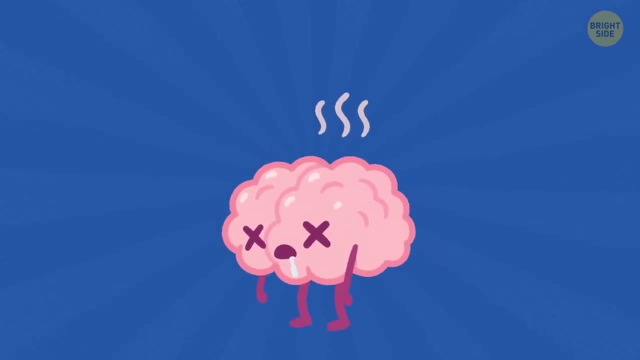 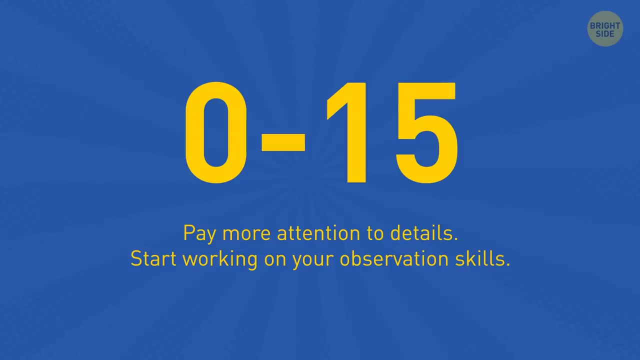 This level has indeed messed with my mind, And now are you looking forward to finding out your results. If your score is 0 to 15 points, you need to pay more attention to small details. As soon as you start working more on your observation skills, your results will get much better. 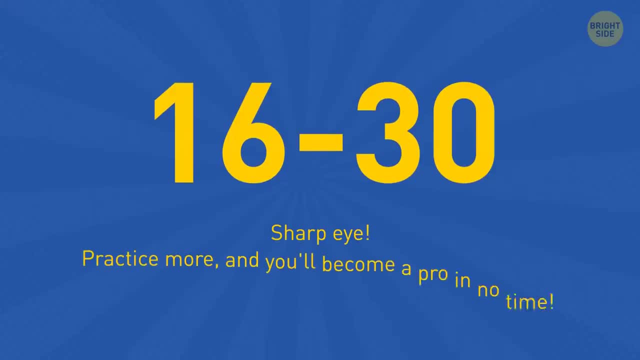 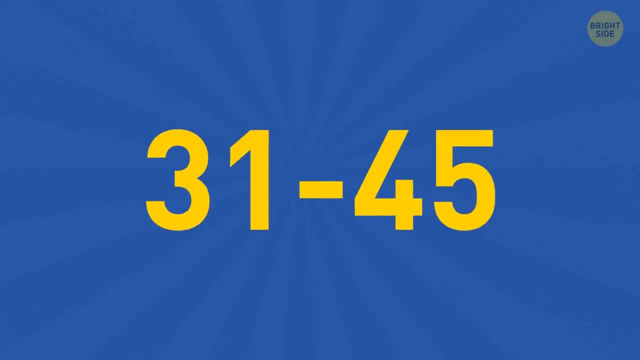 If you've got 16 to 30 points, you have a sharp eye. If you practice more, you'll become a pro in no time. If you have 31 points, you'll become a pro in no time. If you have 41 to 45 correct answers, you can spot the tiniest details and figure out the answers to the trickiest riddles. Nothing can escape your eagle eye.